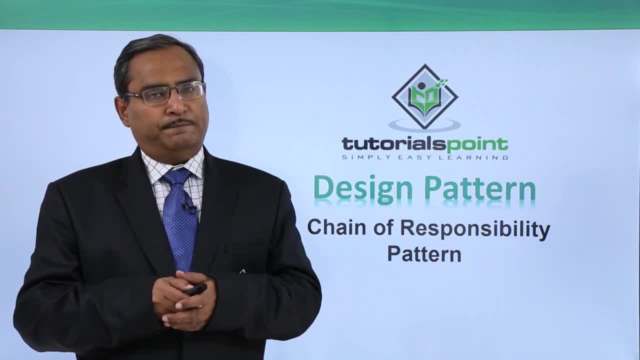 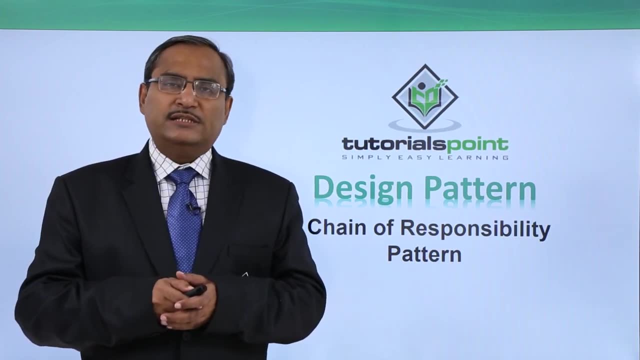 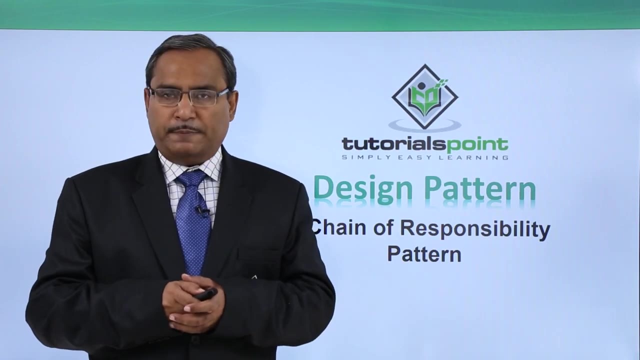 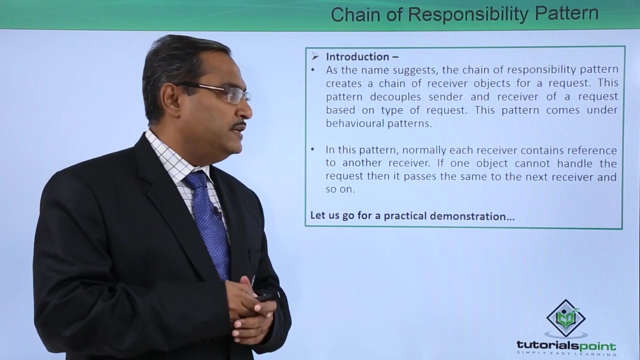 Chain of responsibility design pattern. In case of chain of responsibility design pattern, the change of receiving objects against one request will be created, And this particular design pattern is falling under the behavioral design pattern category. So, as the name suggests, the chain of responsibility pattern creates a chain of receiver objects for a request. 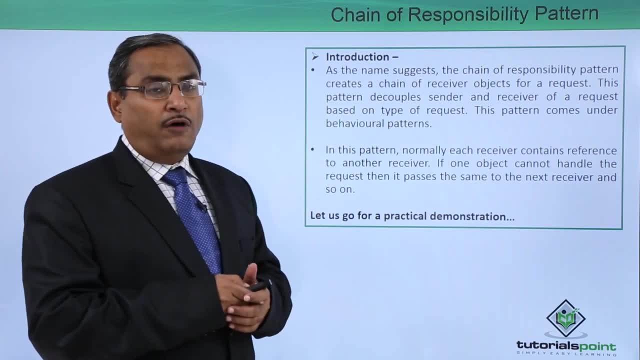 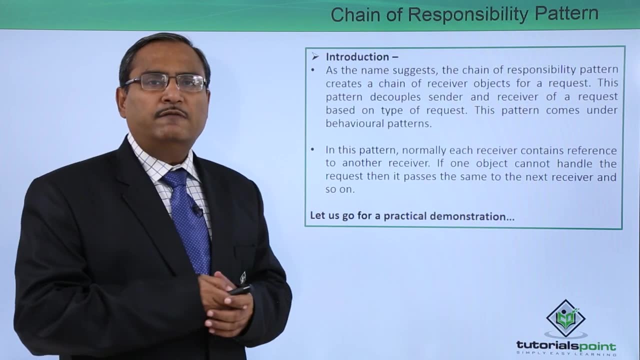 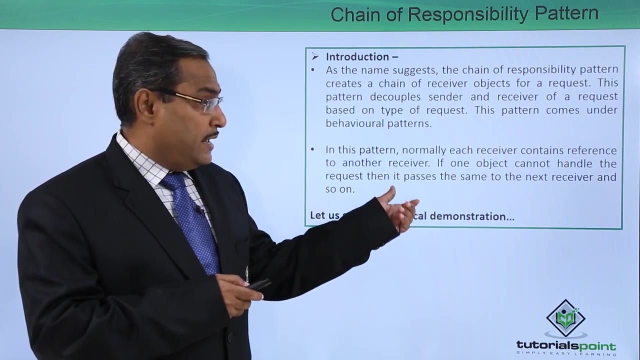 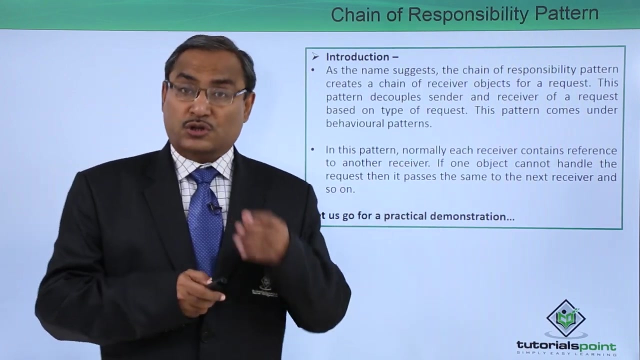 This pattern decouples sender and receiver of a request based on the, depending on the type of the request. This pattern comes under the behavioral pattern, So in this pattern normally each receiver contains reference of another receiver, And if one object cannot handle the request, then it passes the same to the next receiver, and so on. So and that 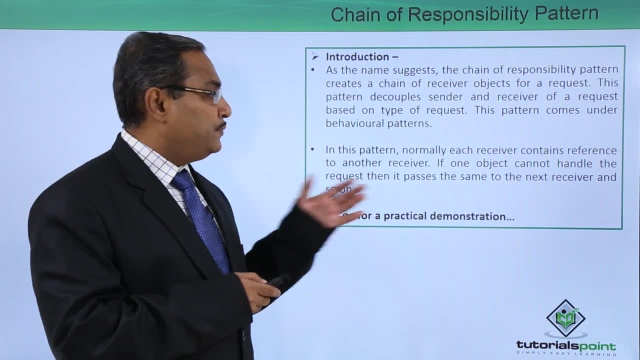 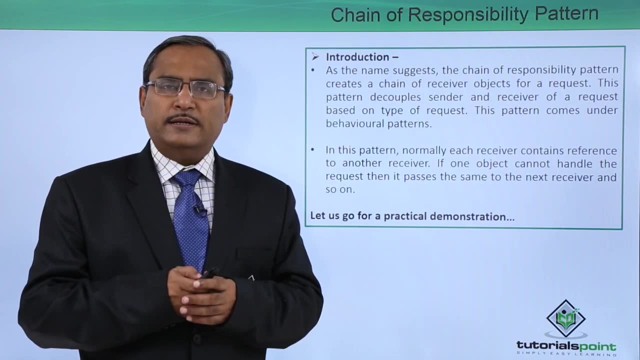 that is why the name of this design pattern is chain of responsibility design pattern. So I think to have a better idea on this respective concept. So let us go for one practical demonstration using Java program and where we will be discussing all this chain. 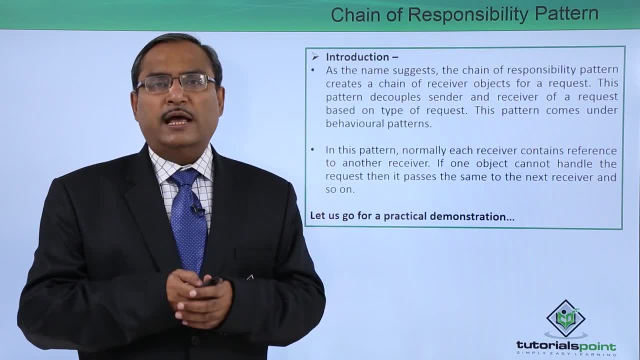 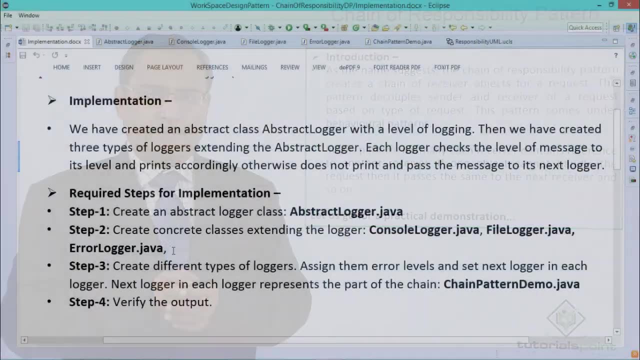 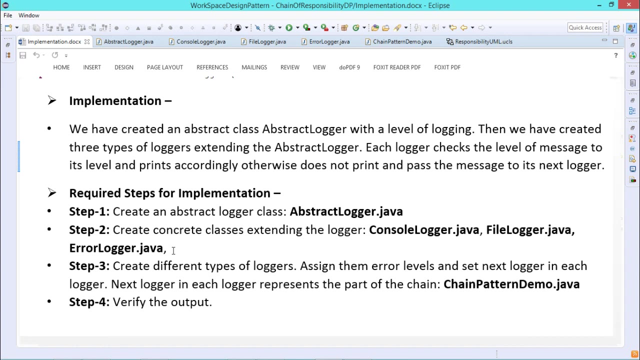 of responsibility design pattern concepts into more details, and it will be supported with UML class diagrams also. So here is the demonstration for you. In this video, we are going to discuss the chain of responsibility design pattern. The chain of responsibility pattern is used to achieve loose consequences. 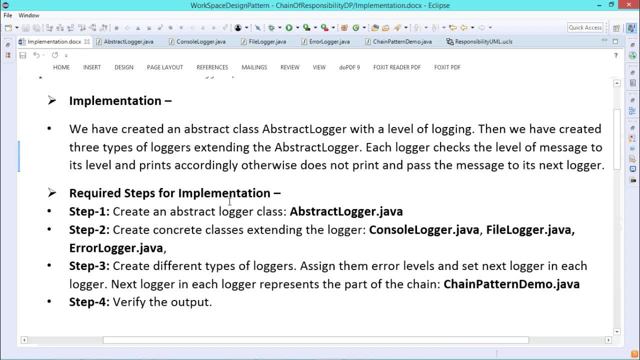 No discipling in the software design. when a request from the client is passed to the chain of objects to process them, Datethet, the object in the chain will decide themselves who will be the processing the request and whether the request is required to be sent to the next object in the chain or not. that is the basic philosophy. 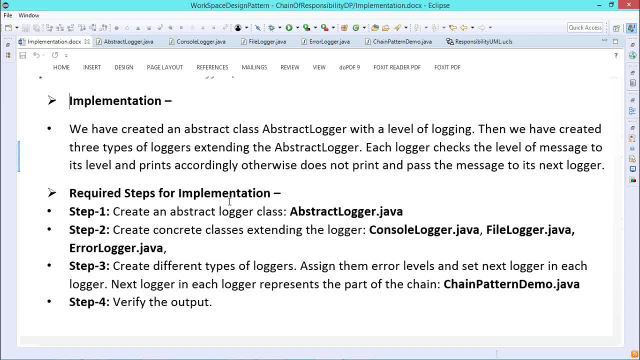 behind this chain of responsibility design pattern. We have created an abstract class here in our case study. As you may know, these are a number only the abstract logger with a level of logging. and then we have created three types of loggers: extending the abstract logger: each logger checks the level of the message and to its level and. 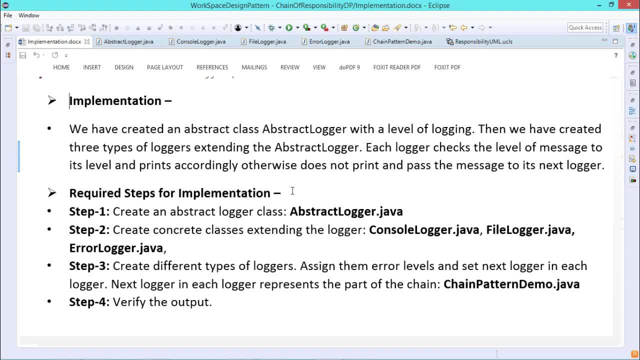 prints accordingly, otherwise does not print and pass the message to the next logger. so required steps for implementation. we are going to implement this case study step by step. at first we're going to have one abstract logger class, that is the abstract logger dot java. so here is the respective 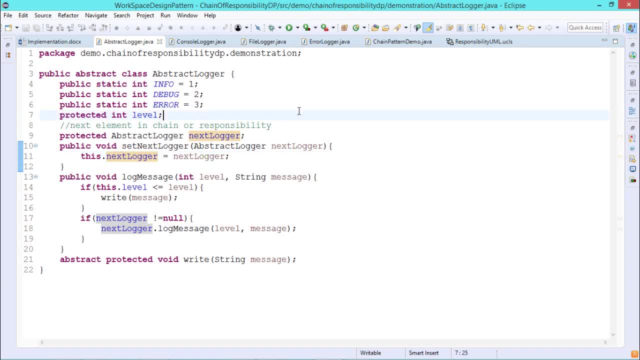 code for us. this is the abstract logger dot java here. you see, here we have defined public static int. info is equal to one, debug is equal to two and error is equal to three. so these are the different levels we are defining and protected int level. so that means this particular level. 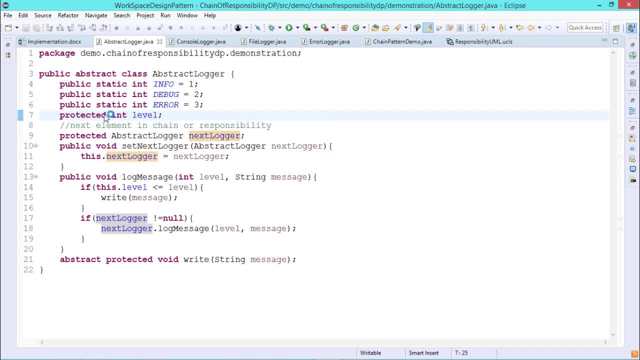 can be inherited because it is under the scope protected. so the next element in the chain of responsibility will be the protected abstract logger object. that is the next logger, so it is also under the scope protected. so public void next logger which is taking this abstract logger class. 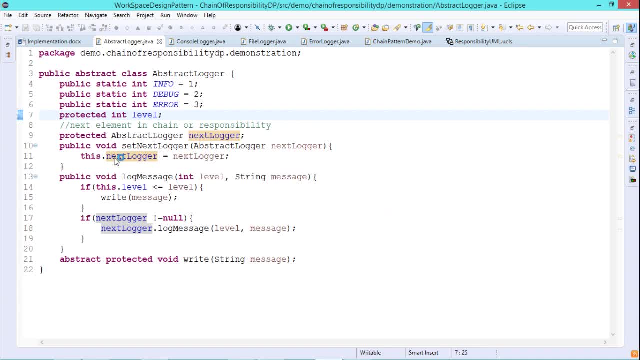 object as input parameter and which is instantiating this next logger with its current object content. so public void. next set. next logger which is taking the abstract logger object as input parameter and which is instantiating the instance variable. next logger. so public void log message. so here we are going. 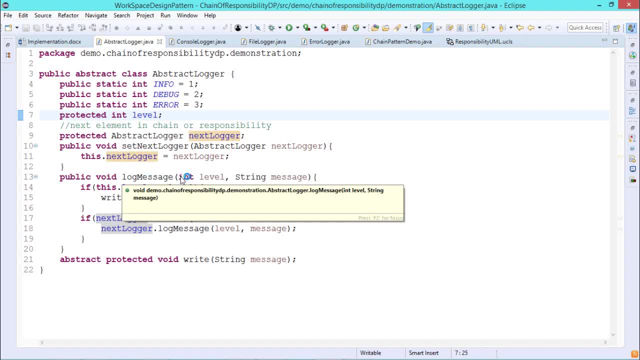 to define another, another respective method, which is having the int level and the string message. so if this dot level is less than equal to level, that means the input argument, input parameter level. if it is greater than or equal to this particular instance, variable level in that case. 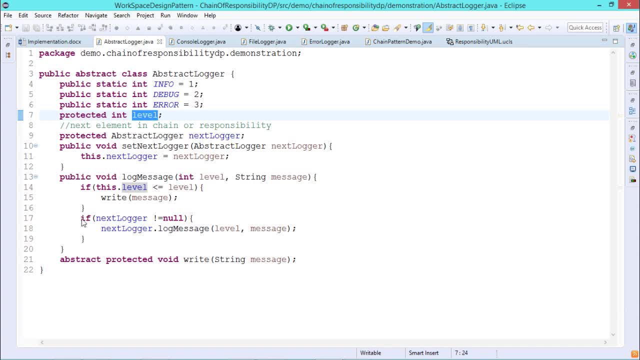 message will be written. so write message and then we are having: if next logger is not equal to null, then next logger dot log message, level message. so if the next next logger is is not null, it is having some object containing some object. so now the next logger dot log message. 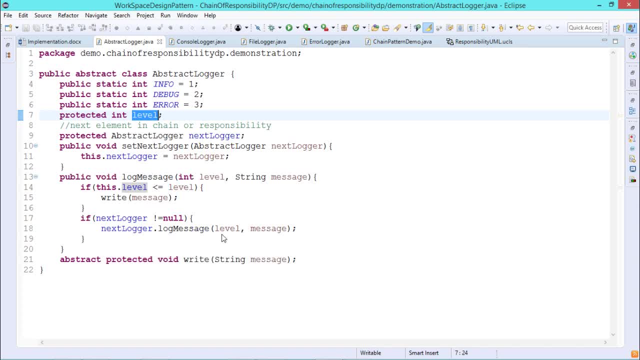 so, again, the log message method will be called from this next logger passing this level and the message here. so here we are having one abstract method that is a write abstract protected void write and string message as it is containing this abstract method. right, so this particular class abstract logger is abstract class abstract logger. so now let us go for the step number two. 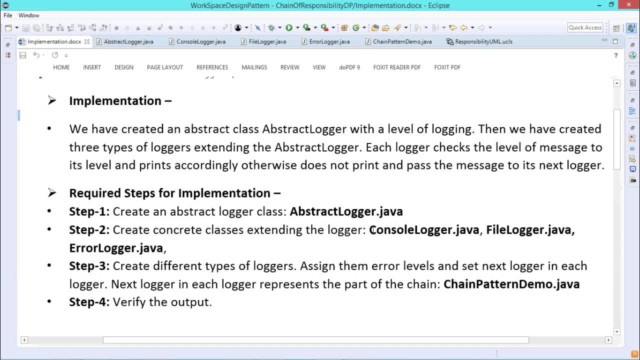 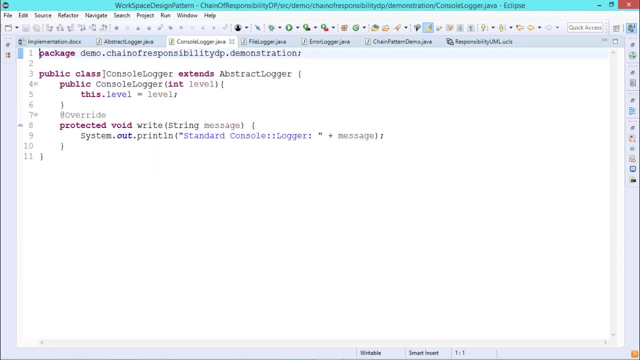 create concrete classes extending the logger. so here we are going for three different classes. one is the console logger, dot java, file logger, dot java and error logger, dot java. so we are going for this abstract logger and then we are going for this console logger, dot java in case of console. 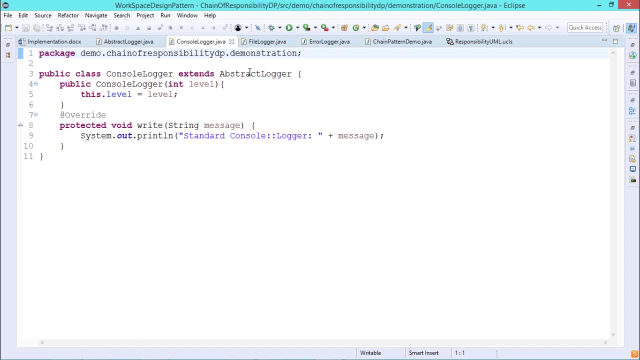 logger dot java, which is extending this abstract class. there is a abstract logger and public console logger. it is nothing but the constructor and it is taking this int level as input parameter and it is just initializing, instantiating. this plot level is equal to level. you can find that this level is under the scope protected, so it is inheritable. so from this console. 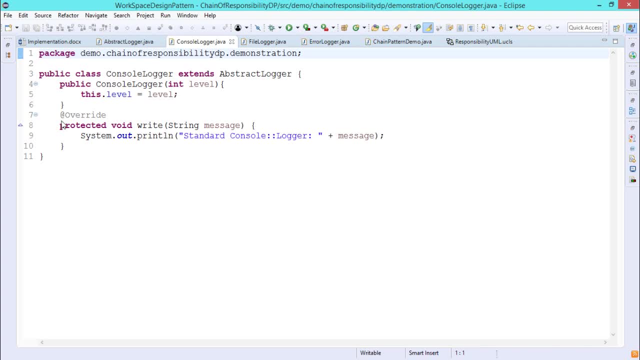 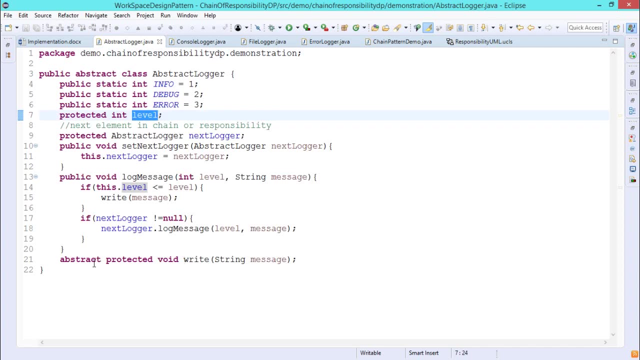 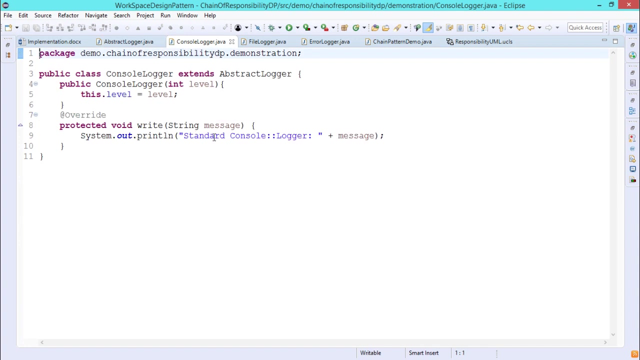 logger. this level can be accessed when having this particular method, that is, the write. this write method is going to get overridden here. so here you see. this write method was abstract, protected void write string message. so we are defining this write method body so which is printing this required statement, concatenating it with the message here now, similarly, we are 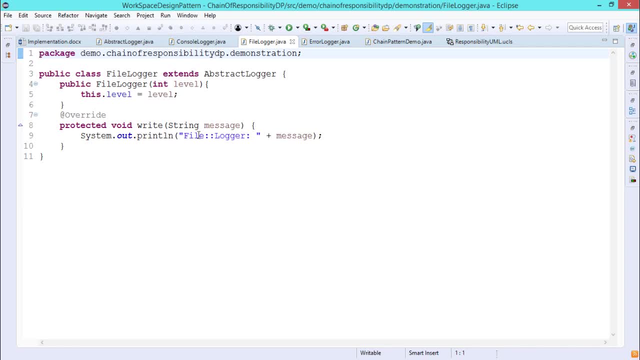 having this file logger. you can have the same type of code. but here we are having this five colon colon logger, colon concatenation message. we are having this error logger. error logger is having the same kind of code, so everything is same. only here this particular message is got changed. 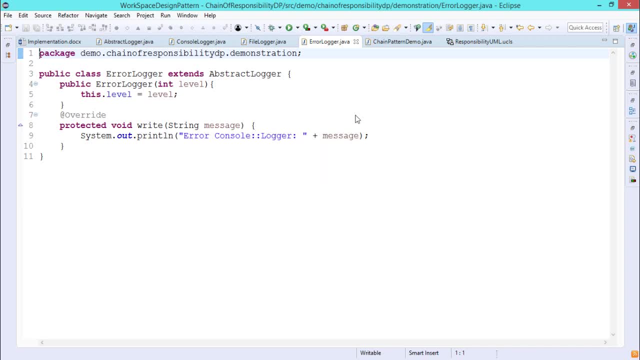 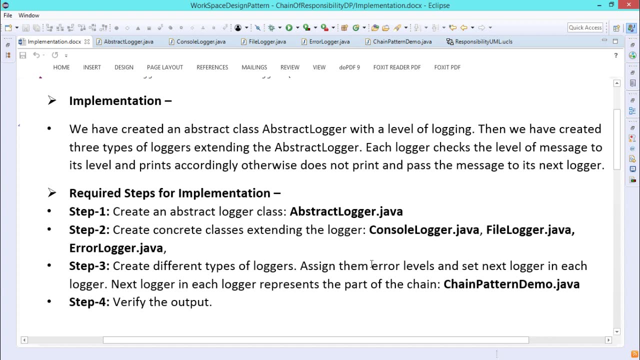 colon, colon logger, colon concatenation with this message. now we're coming to this step number three: create different types of loggers and assign them, assign them error levels and set next logger in each logger. and next logger in each logger represents the part of the chain and that has 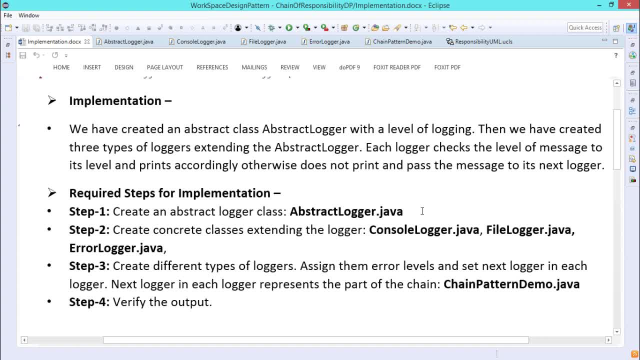 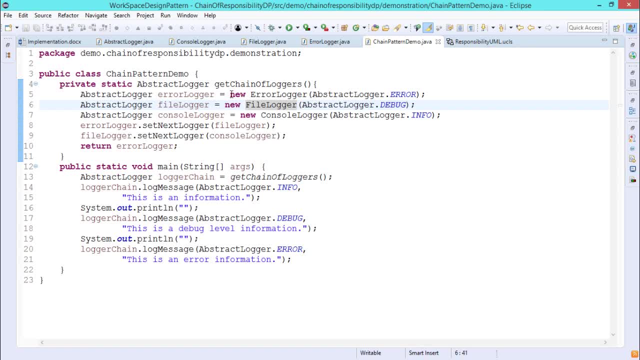 been implemented in this chain pattern: demo dot java class. so let us come to this chain pattern. so here we are defining abstract logger. error logger is equal to new error logger, appster logger. abstract logger, dot error. we know that error is having the value 3. here you can easily find that. 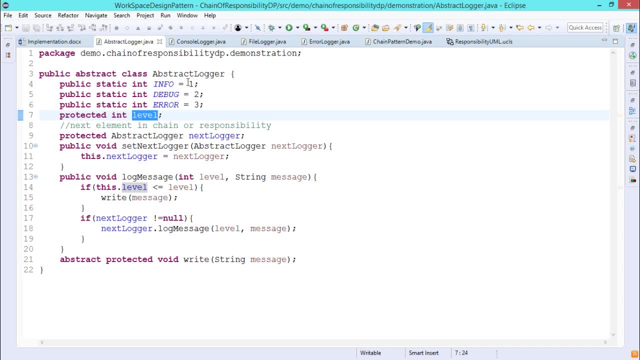 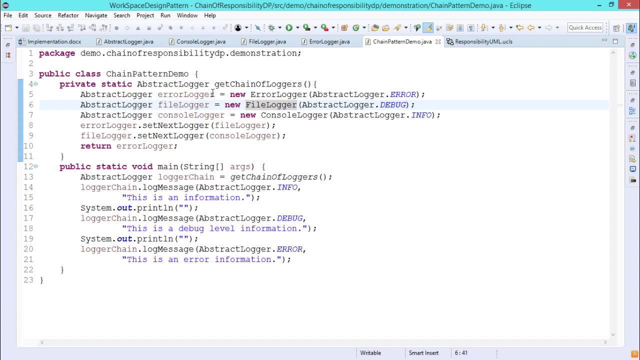 error is having the value 3, debug is having the value 2 and info is having the value 1 here. so now here, in this way, we are going to define this abstract logger object, that is the error logger. similarly, we are defining abstract logger uh, abstract class object, that is a file logger. 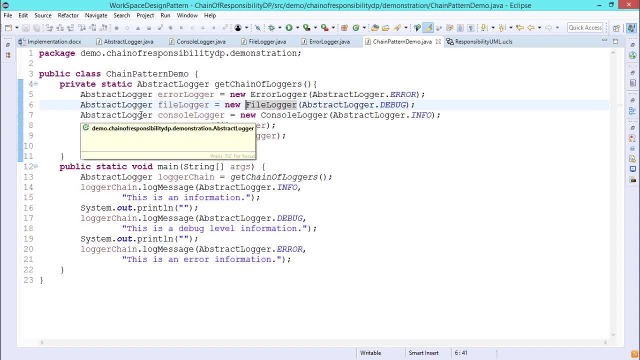 and also we are defining this abstract logger, abstract class object, that is the console logger, in all the cases we are just calling the error logger constructor here new error logger, abstract logger, dot error. so the three is being passed to put it in the level, and then new file logger. so 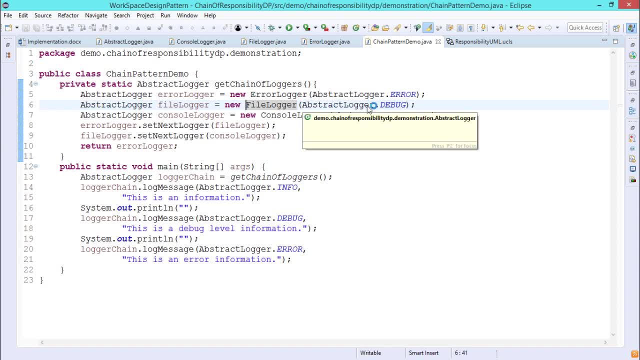 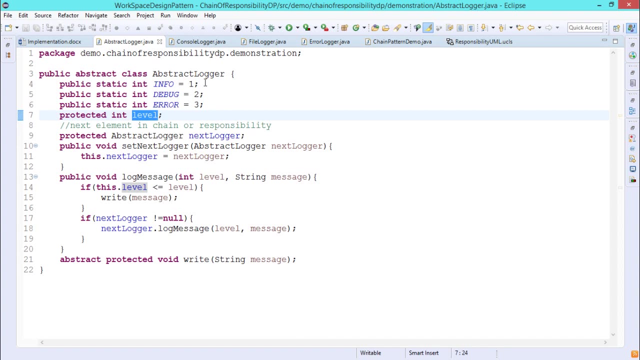 abstract logger dot debug. so two will be the value here and that has been passed as input argument to to instantiate that level. and then we're having this new console logger, so error logger dot in four. so error logger dot info is having the value 1 here. error logger dot info is having the value 1. 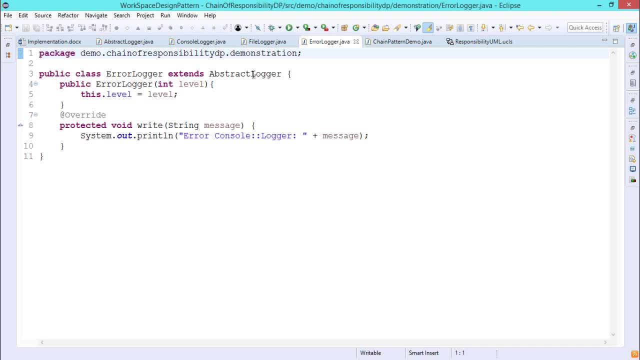 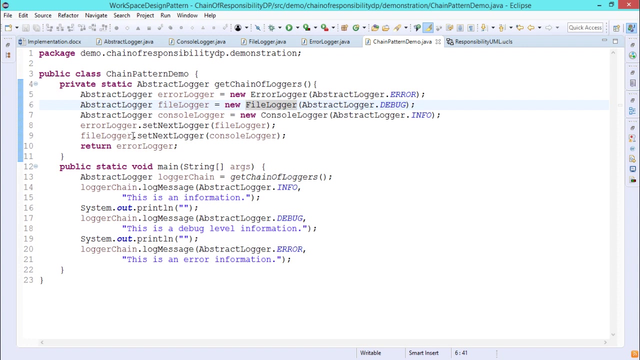 and you know that this is the error logger which is extending this abstract logger. so, whatever the level, i'm passing, that is a 1 which is in in instantiating this dot level. now this error logger is having the set next logger, file logger, and file logger is a dot. 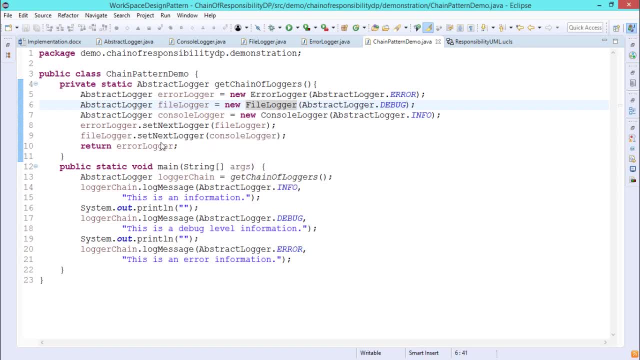 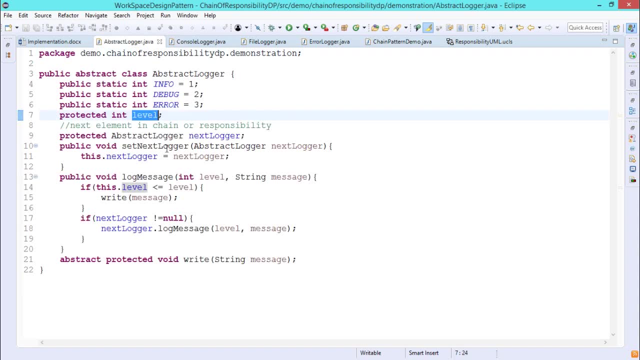 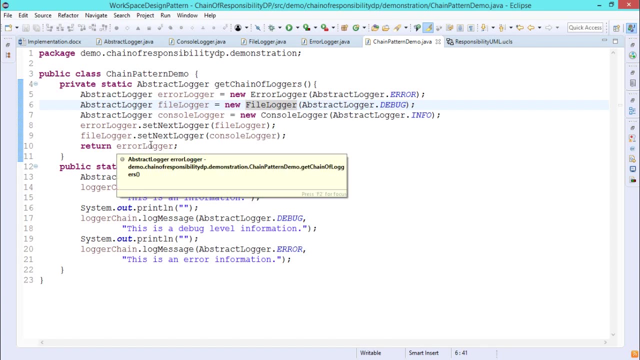 set next logger. that is the console logger and console logger: it's set next logger. i haven't called so. as a result of that, this next logger is remaining uninitialized in case of this particular console logger here. so now return error logger. so error logger will be returned here. okay now. 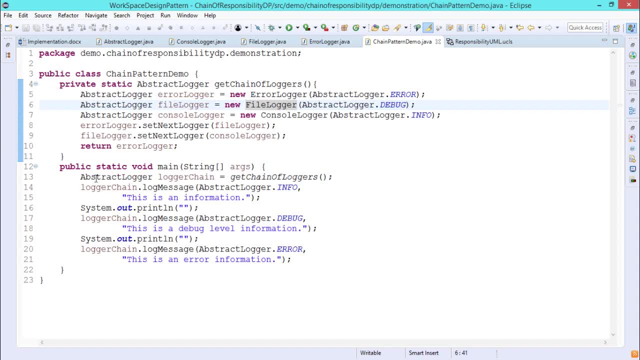 public static void main string args. we are having this, so abstract logger object, that is, a logger chain, is equal to get chain of logger. so this particular method has been called here. this particular method has been called, so as a result of that, it is returning the error logger, so error. 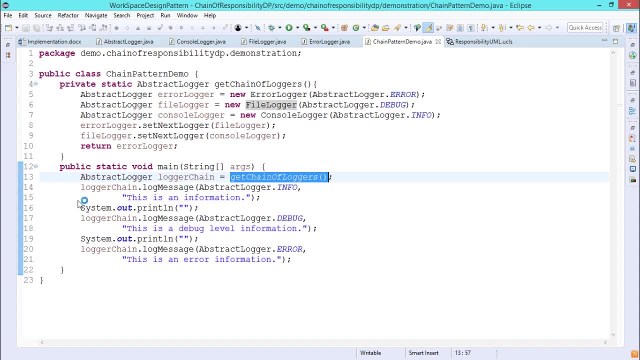 logger is is being assigned on this logger chain. so logger chain dot log message. abstract logger info comma. this is an information abstract logger dot info. this is an information. so abstract logger dot info. here we are having the value one and this is an information. is the respective message. 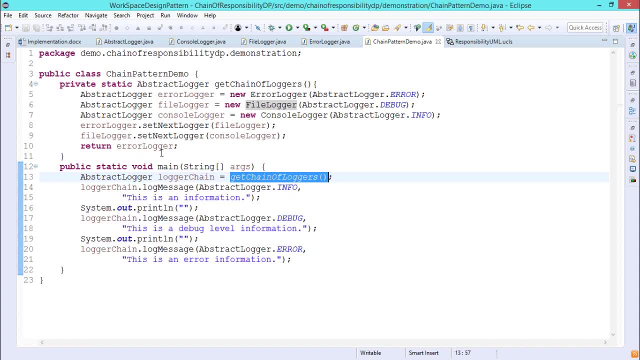 so there is a logger chain which is nothing but the error logger here. so so system dot out, dot println. i'm just putting one null string here only to break the continuity. so let us put the output side by side for the better understanding. so here we are having this. 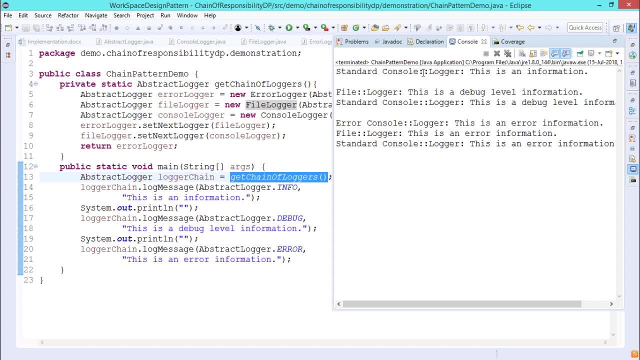 output here. so there is a standard console. colon colon, logger colon. this is an information. so here you can find that here we are passing this: get chain of loggers and logger chain dot. log message, abstract logger dot. info and info. you know that info is having the 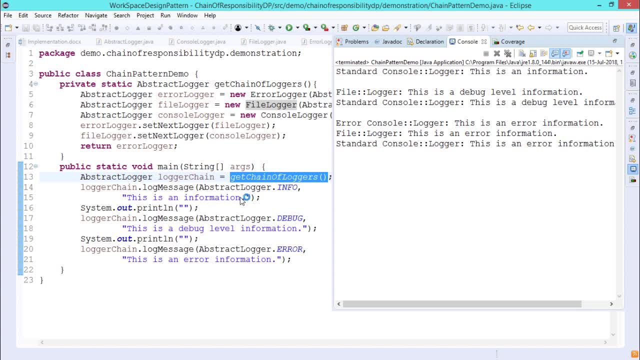 value one and this is an information. so, as a result of that, and this is the value one we are having, so as a result of that, we are getting this required output has got printed and you can find we can. is we can we know that this console logger is having no next logger instantiated. next, we are. 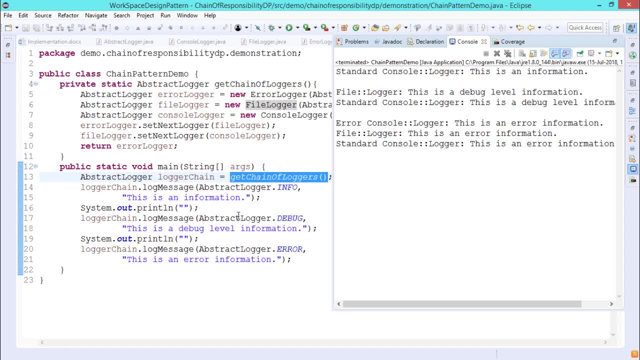 having this logger chain dot log message, abstract logger dot debug. so here this particular value is, here the value is two and this is: this is a debug level information. so what is happening? you can find that file, colon, colon, logger colon. this is a debug level information. so that message. 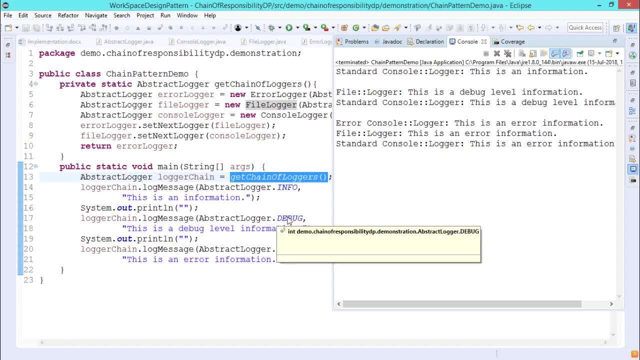 has got printed. so that is our debug here, and this particular debug is having this, that is, the file logger is having the console logger as the next logger. so again we are getting another. another string got printed. there is a standard console colon colon, logger colon. this is a debug level. 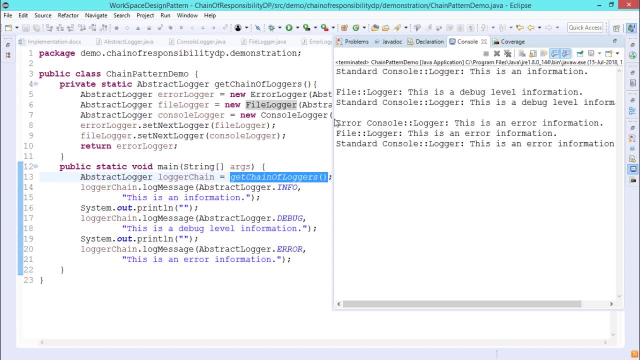 information. so we are having one continuity break here, so that is a continuity break. now, here we are having this logger chain: dot log message, abstract logger dot error. so this error is having the value three here. so error is having the value three. so that is a logger chain dot log message, abstract logger. 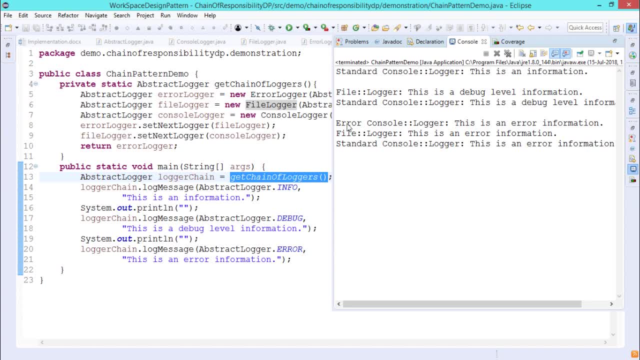 dot error. so it is produced producing the respective message. there is a error console: colon colon logger. this is an error information and its corresponding. its corresponding next logger is our file logger. so file colon, colon logger. colon. this is an error information that has got printed and this file. 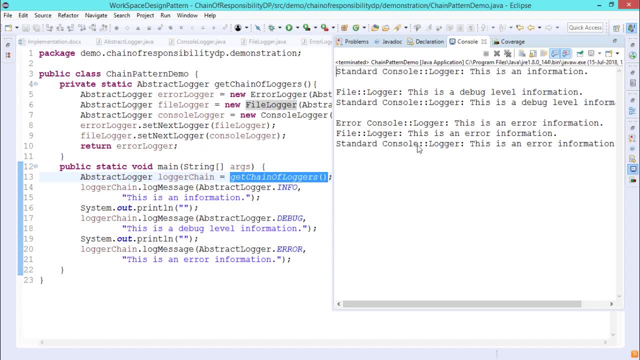 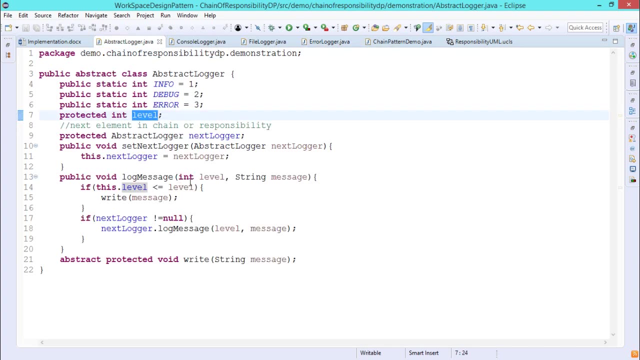 logger is having the set next logger as a console logger. so standard console colon, colon, logger colon. this is an information. this message is getting printed, so we know that whenever the printing is coming. so it depends upon this respective fact that whether this particular level which has been passed as input argument, if it is greater than or equal to the current instance variable. 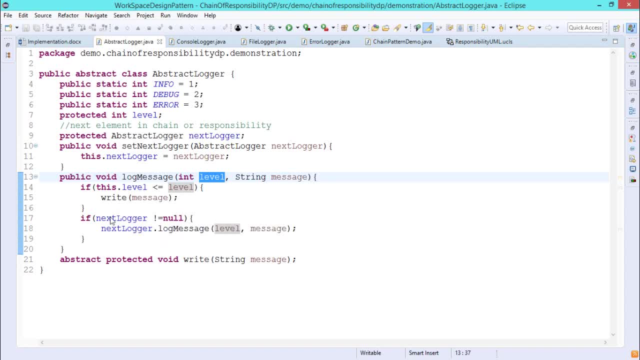 level value, then only the message will get printed, and if the next logger is is not equal to null, then next logger dot log message. this method will be again called so that then it will passing, will be passing this level and the message as the input parameter to this log message. again, the condition: 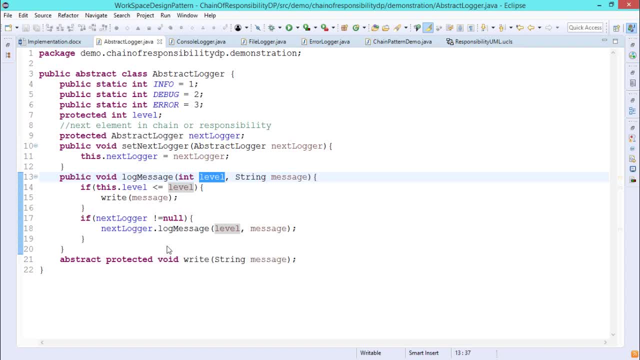 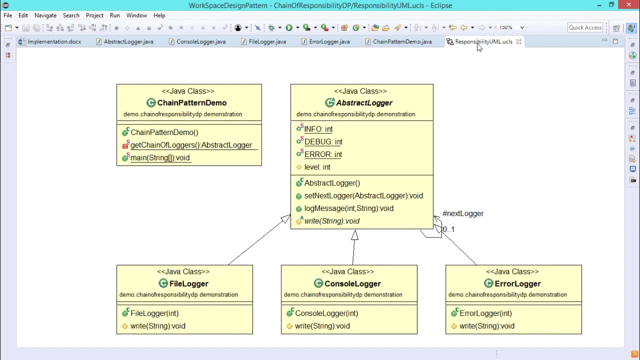 will be checked and again the next logger will be checked, whether it is null or not. so in this way, in this particular demonstration, we have got the idea that how the chain of responsibility design pattern is working and can be implemented using java code. so here we are having the respective 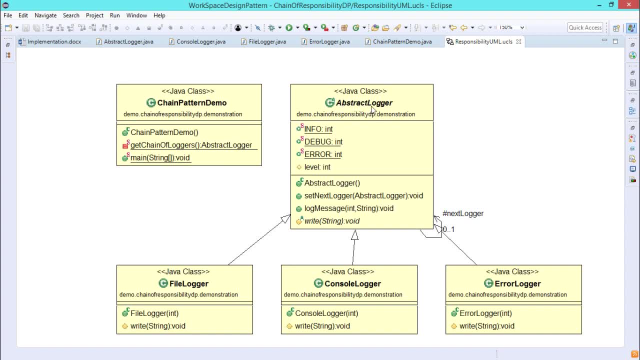 class diagram, the eml diagram we are having here. so abstract logger is nothing but one abstract class here. so there is abstract class and this particular abstract class has got extended to file logger, console logger and the error logger. so file logger, console logger and respective error logger. so here we are having this one and here you see this particular. if you go for this abstract 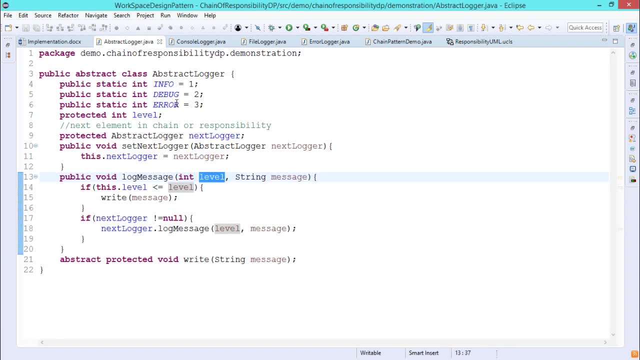 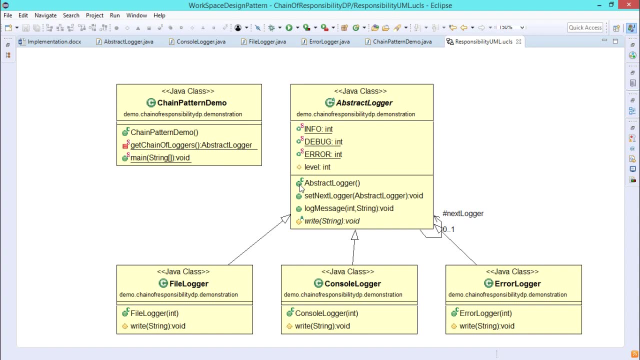 logger. here we are having this info: debug, error and level. so everything has got reflected here. this abstract logger is the constructor under the public section next set. next logger is another public method. this is another public method. that is a log message and this is the right. is there? 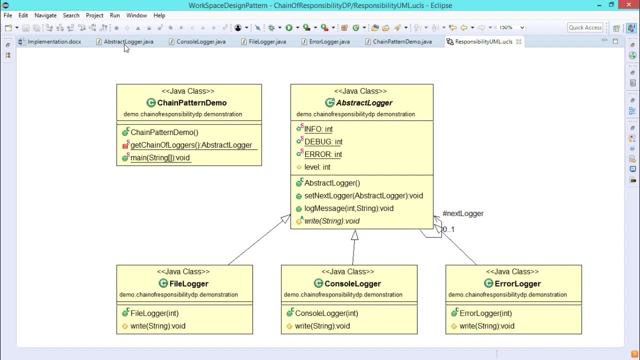 which is the abstract method here, whose body has not been written in abstract logger, abstract class. so there is a right method. okay now, this is our chain pattern demo. this is our chain pattern demo. we're having this chain pattern demo constructor. we're having this static. uh, we are having this, this one, i think. so we're having this static, and this is my private static.